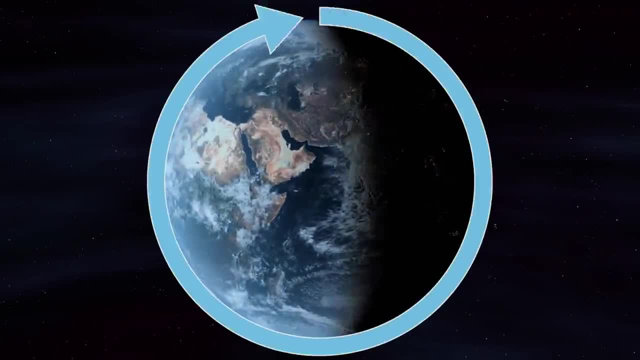 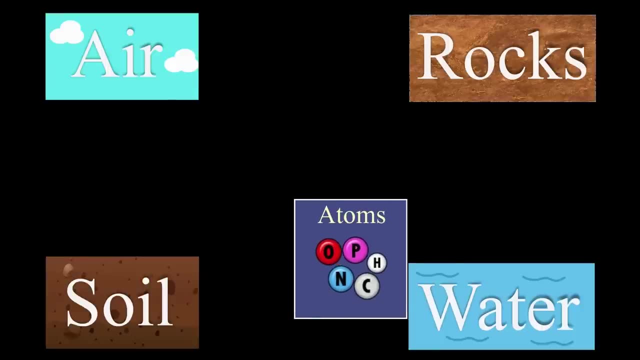 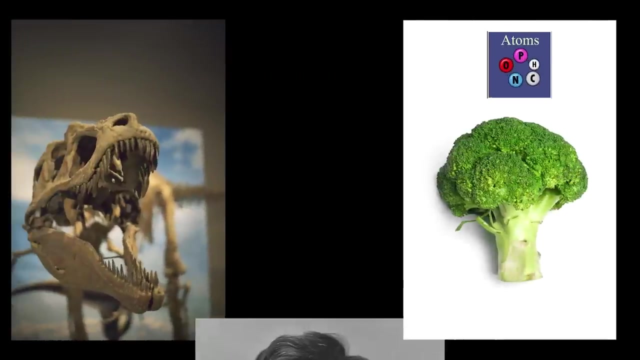 Because the earth is finite, matter has to be reused and recycled over and over again. So the atoms that are in you were once in the air, in soil, in water and in rocks. These atoms have also been used by countless other living things, from dinosaurs to broccoli plants. 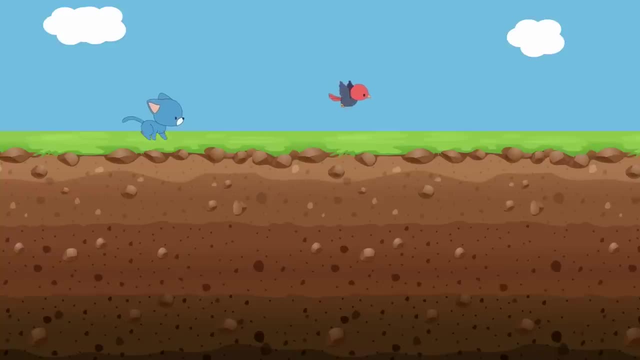 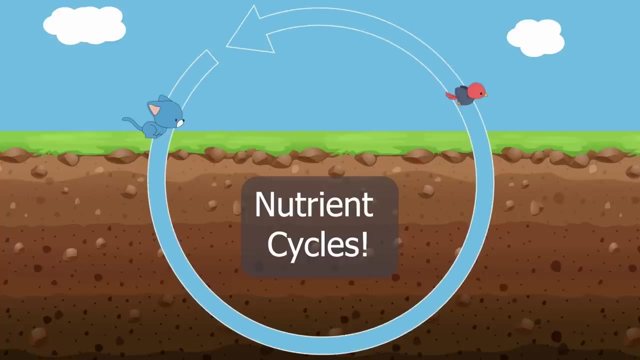 to Abraham Lincoln, And after they leave you, they will become part of other living things or of the environment. This recycling of matter is known as a nutrient cycle, and there are several different nutrient cycles for different elements. Today, we will focus on the nitrogen cycle, the process by which the element nitrogen 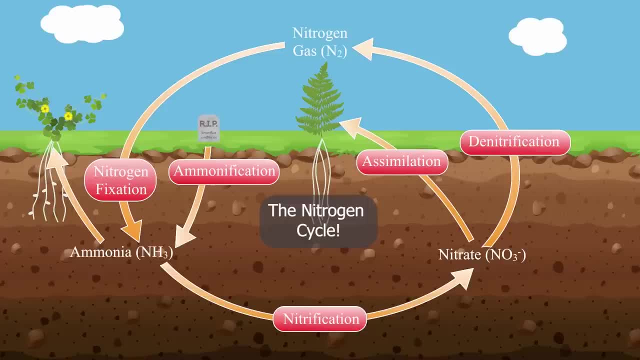 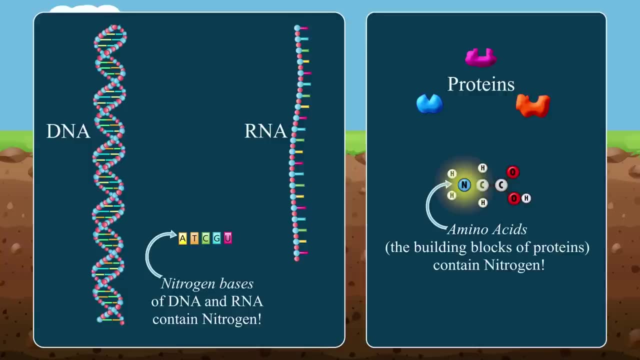 moves around in ecosystems. The nitrogen cycle is crucial for all life on earth, because nitrogen is needed to make some of the most important molecules for life, including DNA, RNA and proteins that are needed by all living things. Without nitrogen, there would be literally no life as we know it. 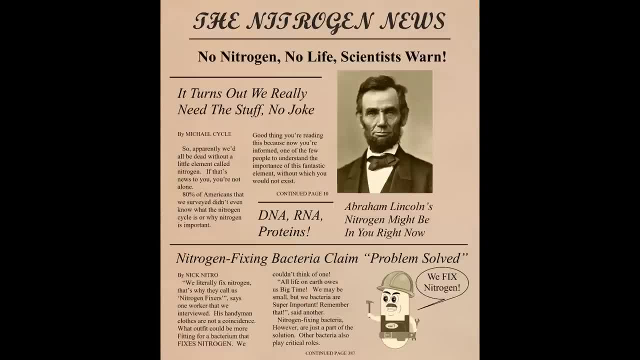 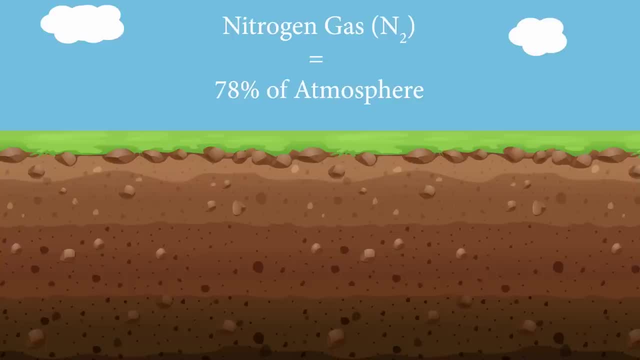 So it's important to understand at least a little bit about how the nitrogen cycle works, right. So let's get into it. Nitrogen gas N2, makes up about 78% of our atmosphere. You breathe it in and out all the 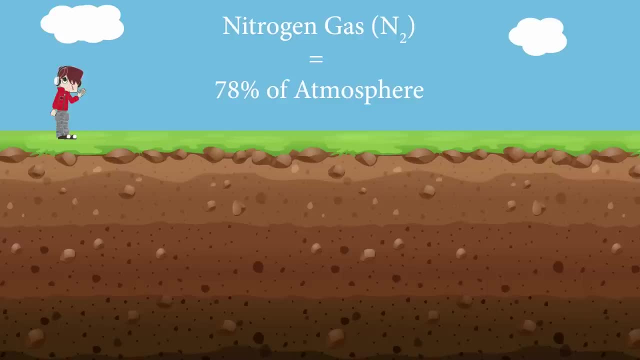 time. In fact, you're doing it right now. The problem with N2 is that you can't use it to make any of the cool molecules we just discussed. The three bonds between the nitrogen atoms and N2 make it very hard to break apart, so you can't use it to make any of the cool molecules we just discussed. 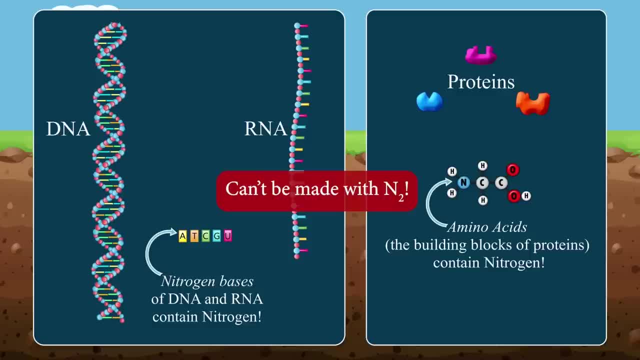 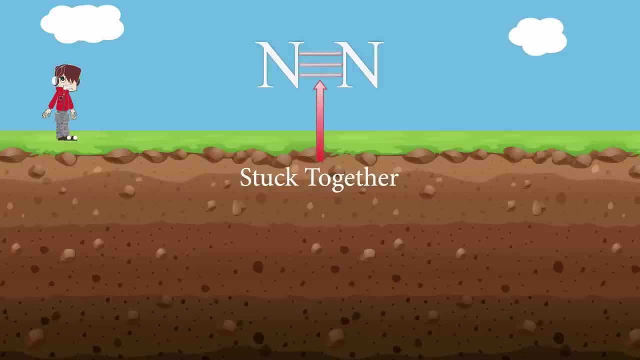 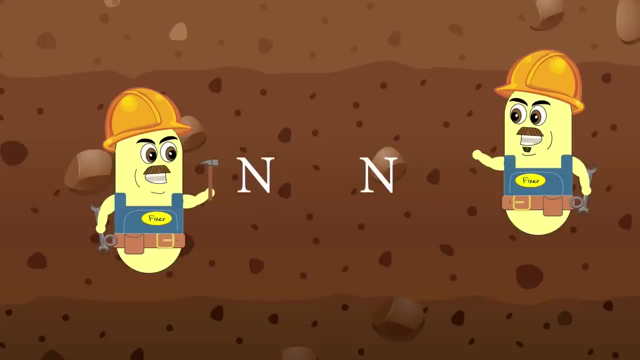 do any reactions to make DNA or RNA or proteins or anything else. The nitrogen atoms are essentially superglued together. Luckily, there are certain bacteria that can break the triple bond of nitrogen gas to make something that organisms can use. These bacteria are called nitrogen-fixing. 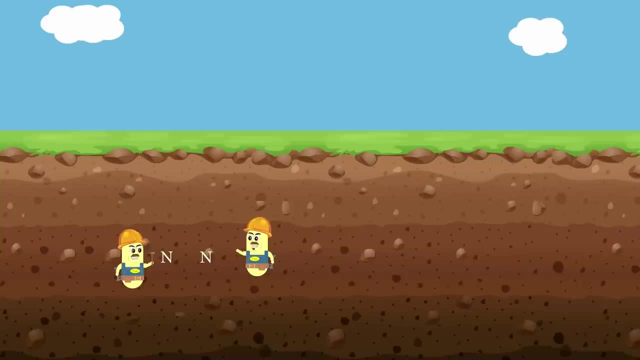 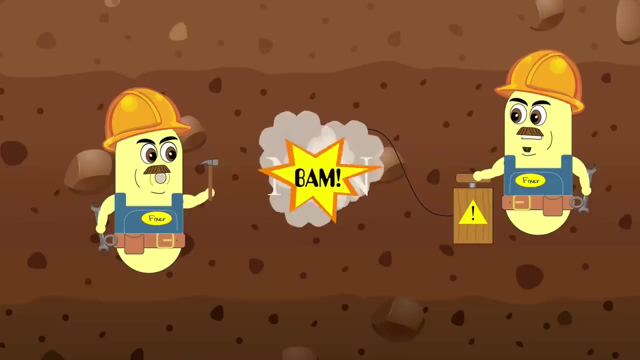 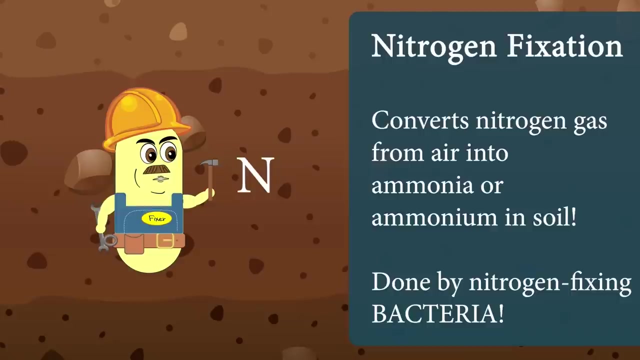 bacteria, and they are found in the soil and in root nodules of certain plants known as legumes, as well as a few other places. These nitrogen-fixing bacteria break nitrogen gas apart and add hydrogen atoms to it to form ammonia, NH3, or ammonium NH4+. 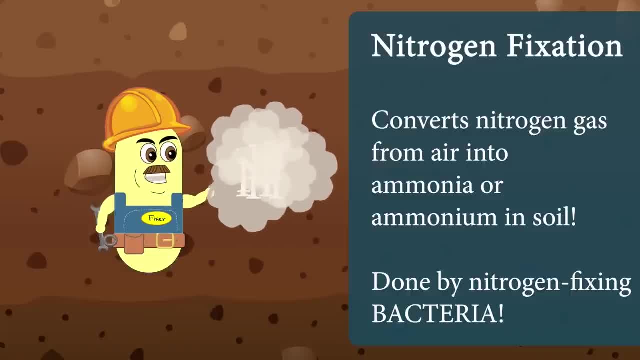 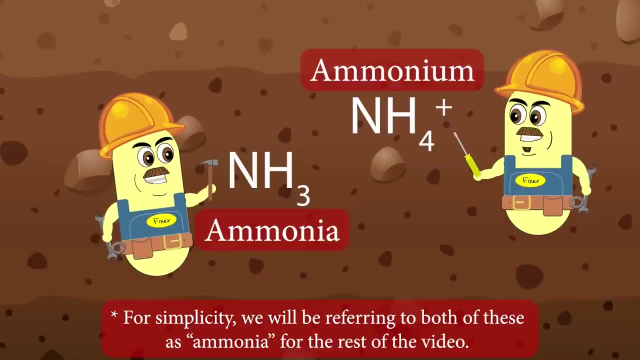 We can fix it. Yes, we can. What's the matter with you? You put another H on there. It's ammonia. It's basically the same, It's just ionized. This process moves nitrogen from the air to the soil. 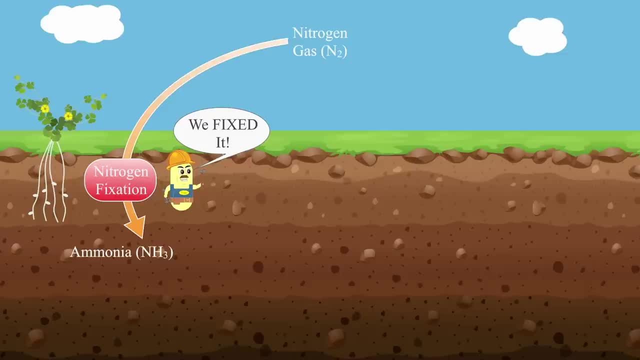 and it's called nitrogen fixation, because the nitrogen in the air is getting fixed so that other living things can use it. Ammonia can be taken up by plants and used to make important biological molecules like DNA and proteins, etc. This process of uptake and 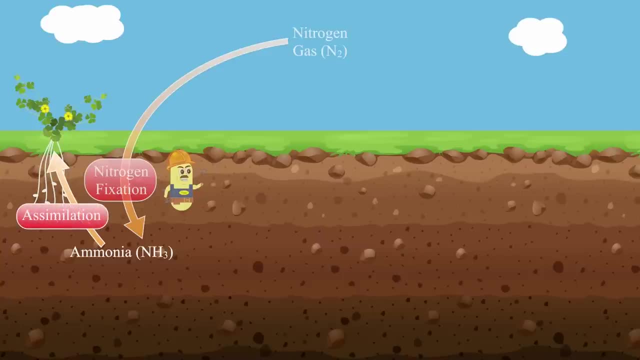 production of biological molecules is called assimilation, But not all of the ammonia produced by nitrogen fixation gets assimilated into plants. Too much ammonia can be toxic and sometimes plants prefer to assimilate it. So if you have a nitrogen fixation, you can use it to assimilate. 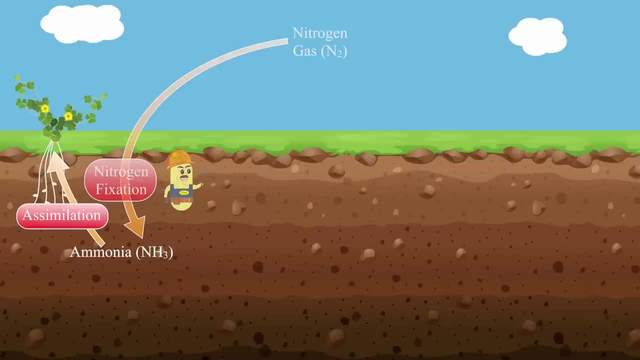 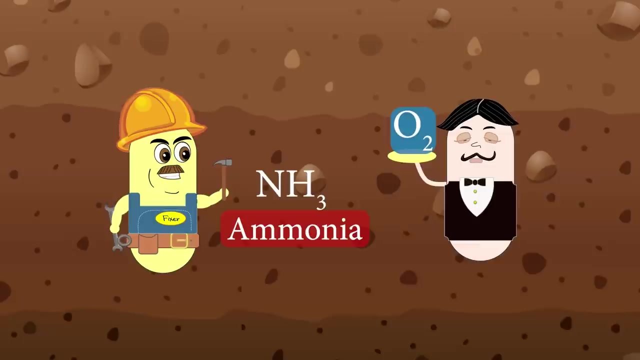 other nitrogen compounds called nitrates. Our next step is the conversion of ammonia into nitrates, a process called nitrification. Hey, we already fixed it. Discerning plants prefer nitrates. Nitrification is done by nitrifying bacteria. These bacteria oxidize or add oxygen to ammonia. 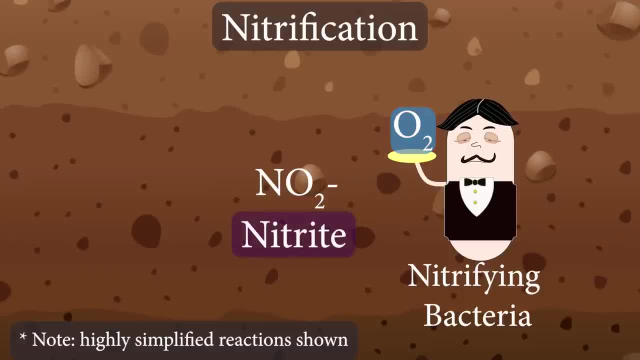 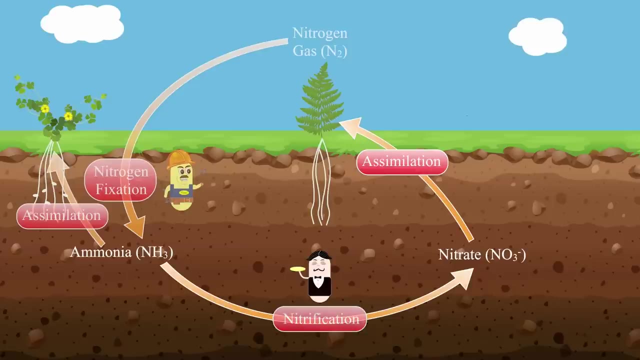 in chemical reactions that first convert the ammonia to nitrite NO2- and then to nitrate NO3-. Because oxygen is needed for these reactions, nitrification happens best in soils that are well aerated. Like ammonia, nitrate is a plant. 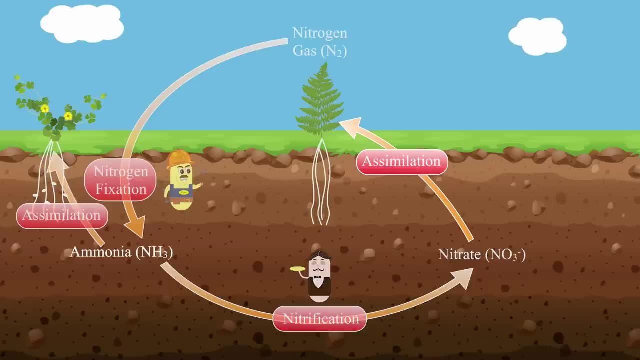 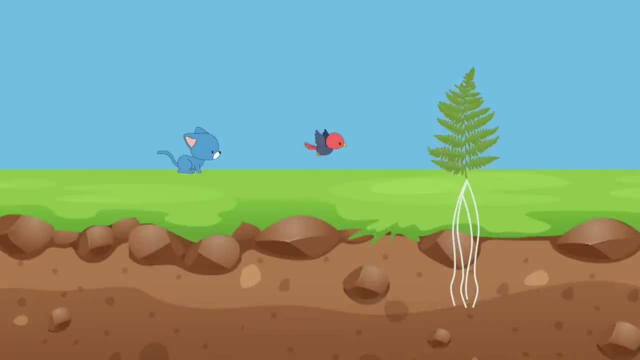 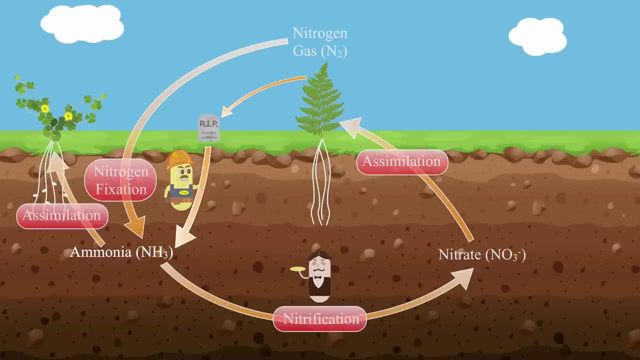 fertilizer because it can be assimilated and used to make key biomolecules, DNA, RNA, proteins, etc. Once nitrogen is inside of plants and used to build our sweet biomolecules, it can pass to other living things through food webs, either in the form of nitrates or nitrification, So by changing nitrogen into a nutrient. 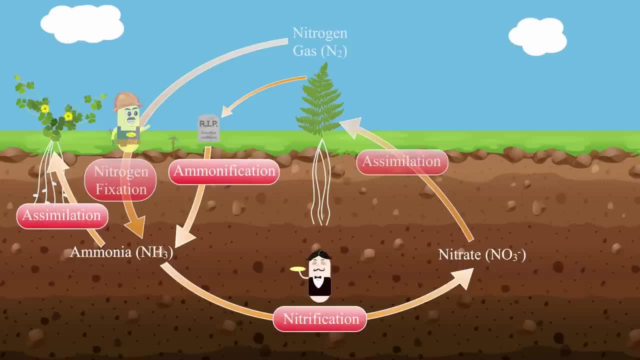 our food webs are in place. When an animal eats the plant, the nitrogen-containing compounds in the plant move to the animal. When that animal gets eaten, nitrogen moves to its predator. Eventually all living things die and decompose. This returns the nitrogen back to the soil as ammonia in a process called ammonification. This ammonia can now be used again by plants or converted to nitrates by nitrification. So nitrogen gets cycled around and around, over and over again. 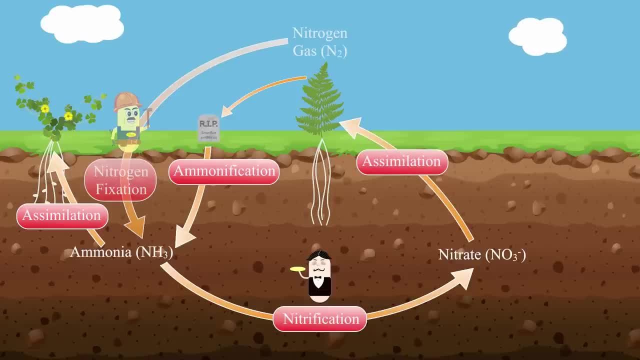 This ammonia can now be used again by plants or converted to nitrates by nitrification. So nitrogen gets cycled around and around, over and over again. We're still missing one key part of our cycle. In order to have a complete cycle, nitrogen gas needs to get back into the air.